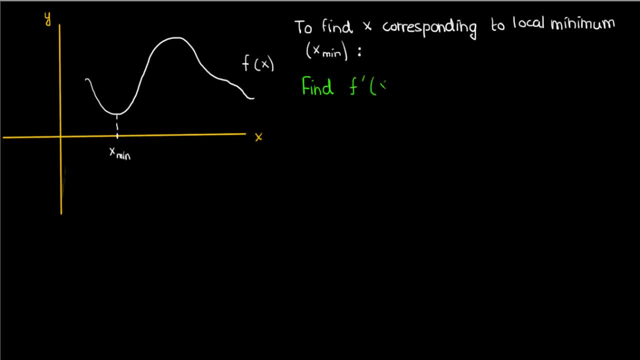 Well, if you remember from calculus 1, then in order to find x min, you start by taking the derivative of the function and setting that derivative to 0. Then the values of x which satisfy f prime, x equals 0, are possible candidates for x min. 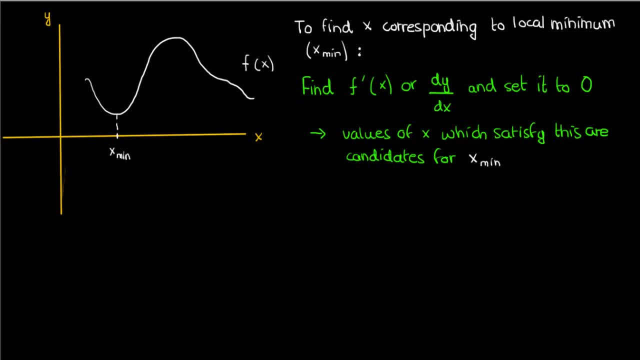 How do you know whether the solutions you get actually correspond to the local minimum? Well, you do further testing by using the second derivative, for example. So setting the first derivative to 0 isn't sufficient to find the local minimum. The solutions you would get to f prime x equals 0 would only be stationary points. 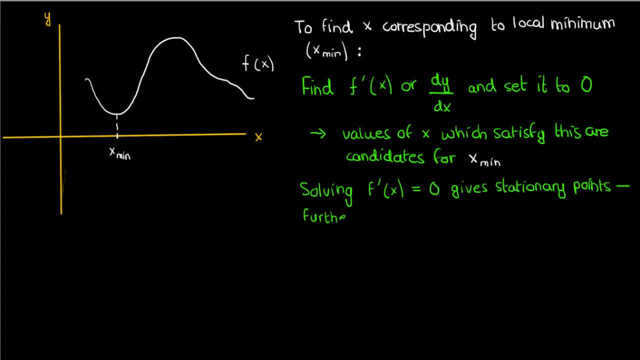 that is, points where the function isn't changing. You would need to do further testing, such as by using the second derivative, to determine the nature of those stationary points. So if we want to find the stationary points of a function f of x, we set its first derivative to 0 and solve. 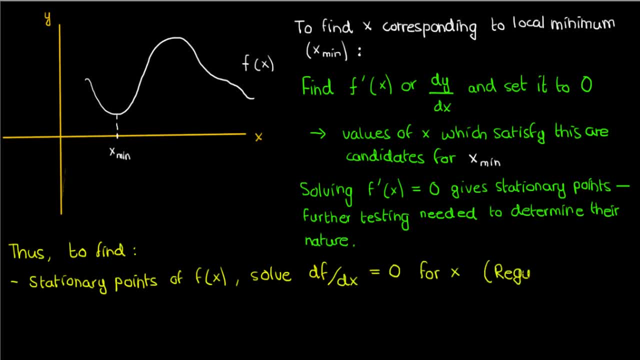 This is, of course, just a problem in your typical single variable differential calculus study. But what if I wanted to go one step further? What if I want to find the stationary functions of a functional that is a function of functions? In that case, what we do is we solve a special equation for the desired stationary function f of x. 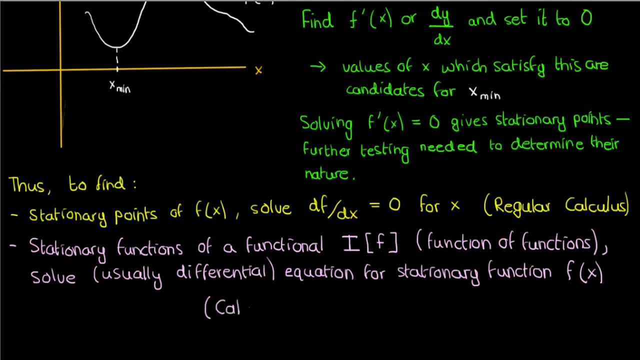 Often this is a differential equation. This second problem is solved using the techniques of calculus of variations or variational calculus, which I'm going to introduce in this video. Now. notice that in going from regular calculus to variational calculus, all I did was add an additional layer of function to my problem. 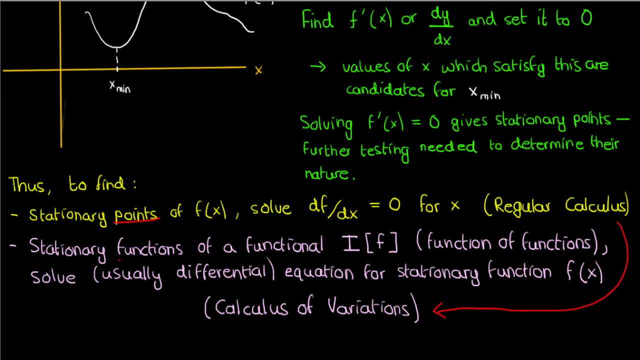 The stationary points from regular calculus now become stationary functions. the function becomes a functional and the equation to solve for the stationary points becomes an equation to solve for a stationary function. You might still be confused about what calculus of variations is all about. 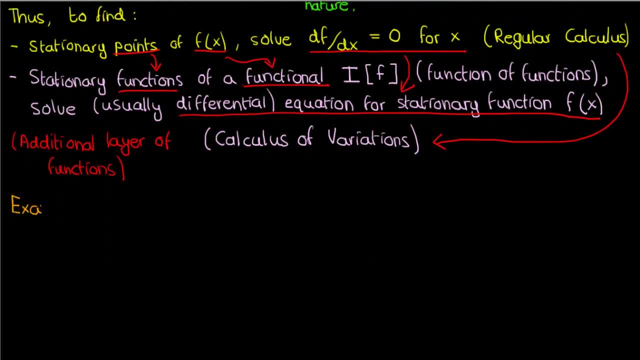 so let me explain things with an example of a typical problem you'll see in variational calculus. Suppose I have two points on the xy-plane, a given by x1- y1 and b given by x2- y2.. Now what I want to do is find the path linking a and b such that the distance between a and b along that path is minimized. 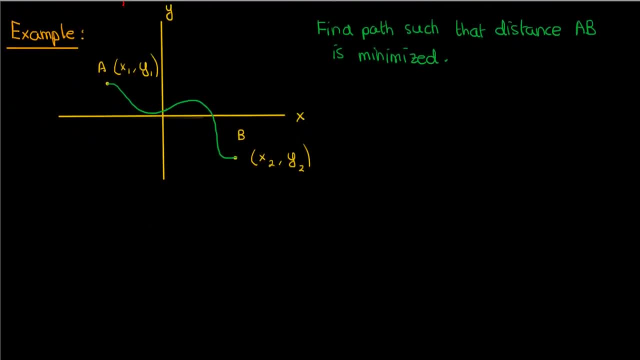 This might seem like a trivial problem because obviously the path which minimizes the distance a- b along a plane is just a straight line linking a and b. But let's formulate this as a calculus of variations problem to give you a better idea of what we'll have to deal with in this lecture series. 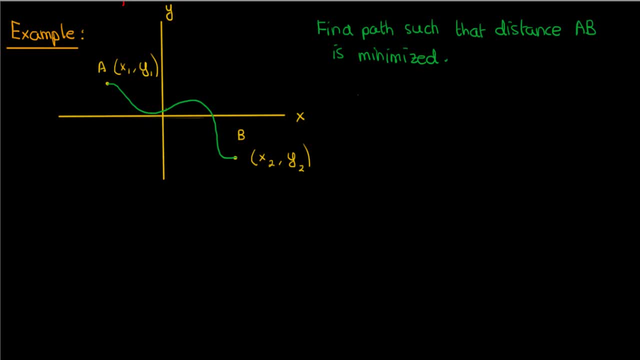 You know from calculus that the length of a smooth curve y equals f of x between two points a and b. I'll call that length- i is just given by this arc length formula- the integral from a to b of ds, where ds is just an element of arc length. 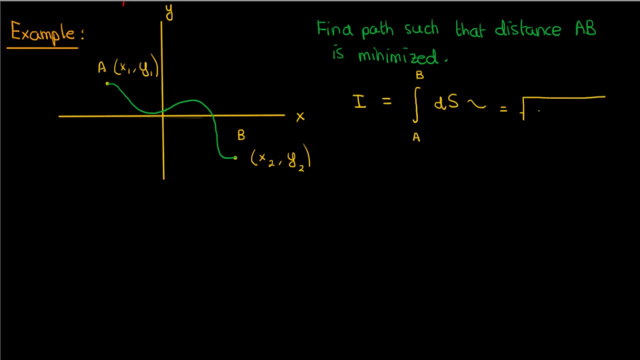 If we use the Pythagorean theorem, then ds is just the square root of dx squared plus dy squared, where dx and dy are just small distances in x and y. If we take out the dx, then we'll get the following, And if we plug this into i: 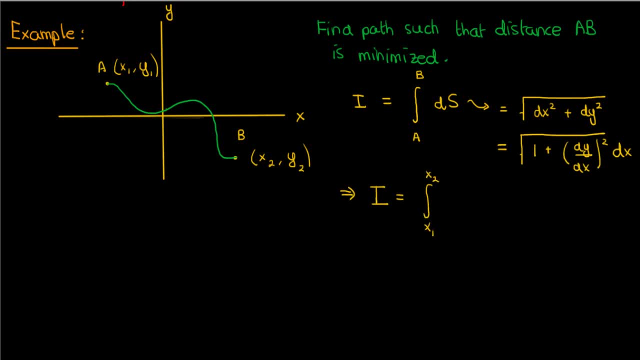 then we'll get the integral from x1 to x2 of the square root of 1 plus dy by dx squared dx. Now, since we want to find the path, and by path I mean the function f of x, the y, Since we want to find the path of minimum distance. 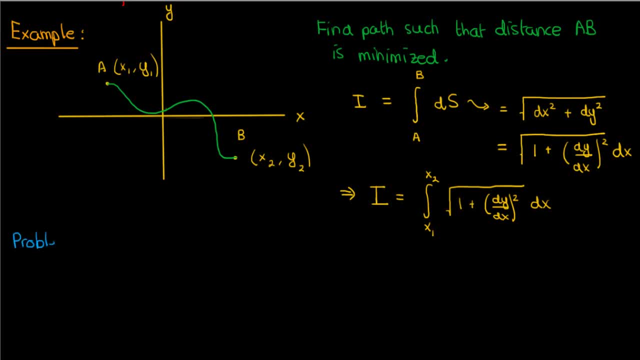 we can formulate a calculus of variations problem that looks something like this: Find: y equals f of x, our stationary function between the points a and b, such that the integral i from x1 to x2 of the square root of 1 plus dy by dx, whole squared dx is minimized. 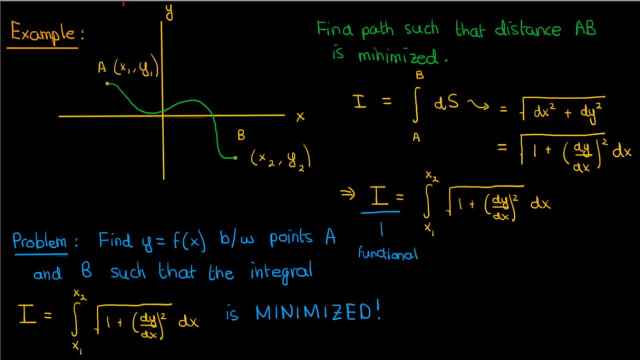 In this case, the functional we want to minimize is i, and what we're minimizing with respect to is the function y equals f of x. Generally, we aren't always minimizing the distance between two points. We could be minimizing a multitude of other quantities. 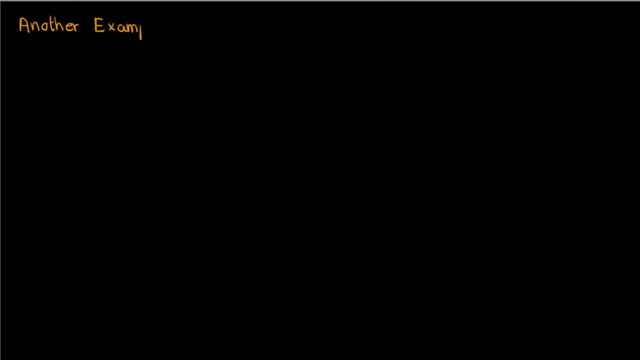 and we could even be maximizing something. For instance, suppose again that we have two points, a and b. Suppose also that we know the velocity of a particle as a function of the coordinates x and y. What we want to do here is find the path- y equals f of x- such that the time taken by the particle to travel from a to b is minimized. 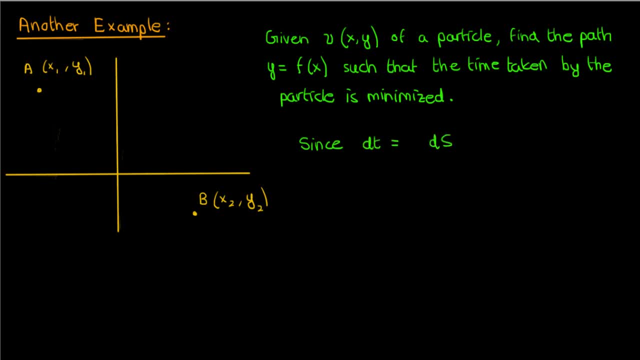 Since the time element dt is just the distance element ds divided by the velocity v, the total time taken to travel from a to b is given by the following integral: If the particle is falling in gravity along a path connecting points a and b, then this problem has a special name. 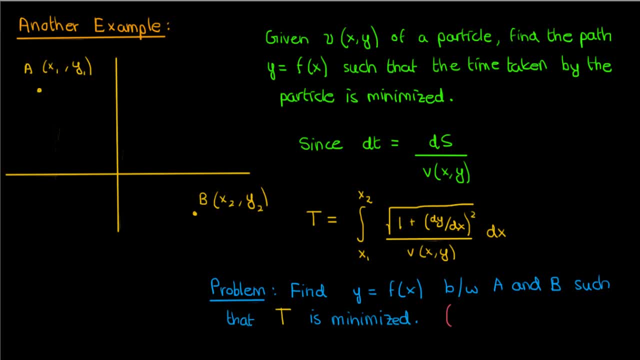 It's called the Braque-histochrome problem. So hopefully these two examples give you an idea of the problems that calculus of variations deals with. In general, the idea of calculus of variations is to find a function f of x that makes this integral of a particular function y equal to x. 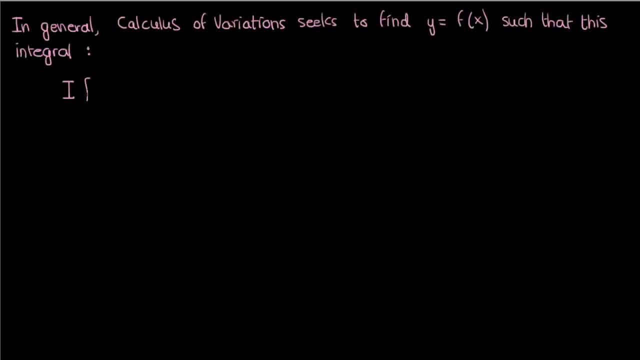 So in this example we're going to find a function y where the integral is 0, plus dy equals f of x, which is the number of the points b and b, the length of the particle. and also we also have the function y equals f of x. 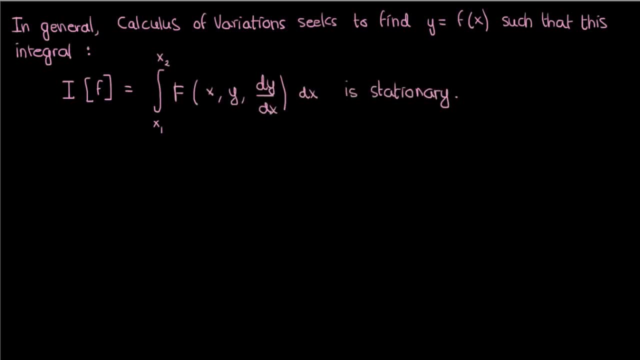 Then we're going to find the function: y equals f of x, which is the number of the points b and b stationary. You can verify that. the two examples I gave fit this general pattern. Note that this capital F is just an expression involving x, y and dy by 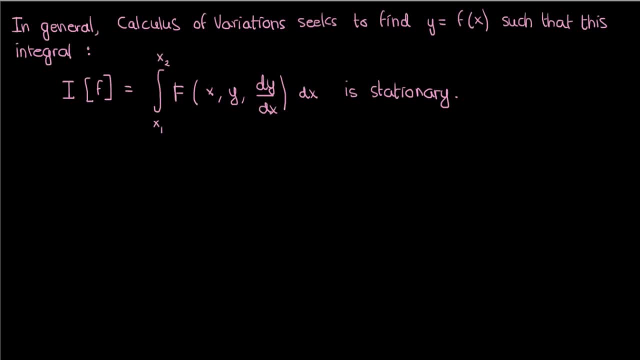 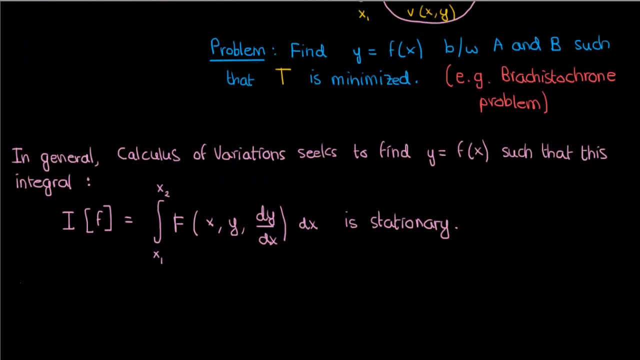 dx. If you use different expressions for capital F, you'll end up with different functionals. For instance, if you use this as the expression for capital F, you'll end up with the time functional. Anyway, that's going to be it for this video. I. 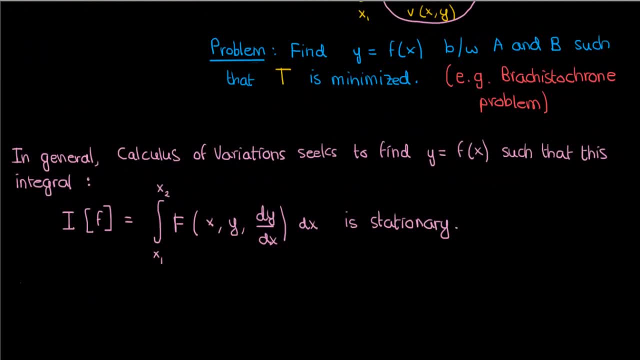 hope it gave you enough of an idea of what calculus of variations is all about. In the next video I'm going to derive the Euler Lagrange equations. The Euler Lagrange equations are basically the variational calculus analog of the F primex equals 0, equation used to find the stationary points of a function. 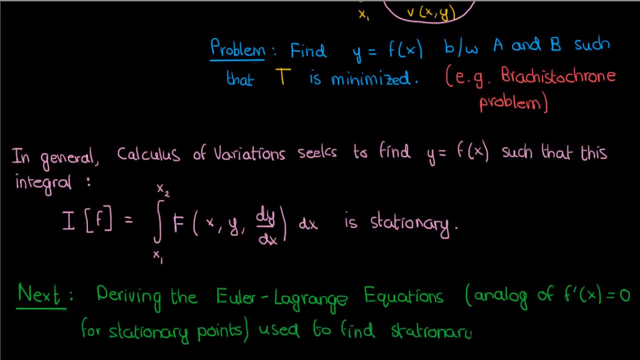 Euler Lagrange is used to find the stationary functions of a particular functional. Just to note. the Euler Lagrange equations don't tell you the nature of that stationary function. they don't tell you if it minimizes the functional or if it maximizes the functional. 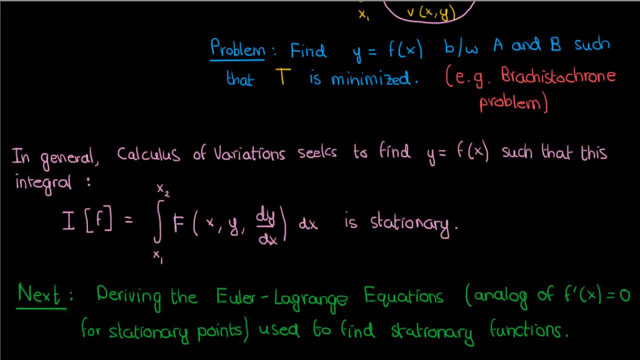 It just tells you that it makes the functional stationary, so it doesn't tell you about the nature. Just keep that in mind. So that's it. If you have any questions, please ask in the comments and if you enjoyed the video, feel free to like and subscribe. Thanks for watching and this is the Faculty of Hans signing out.